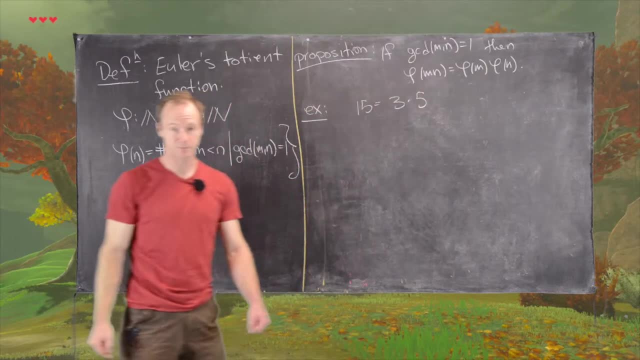 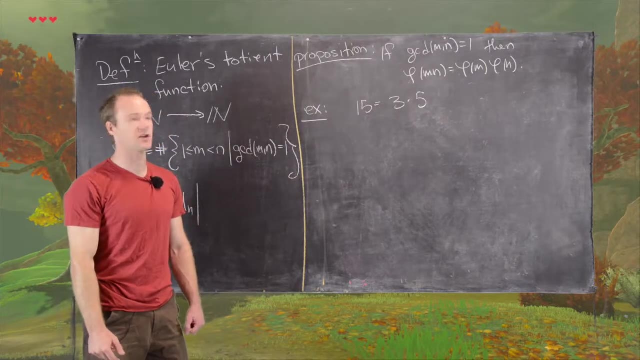 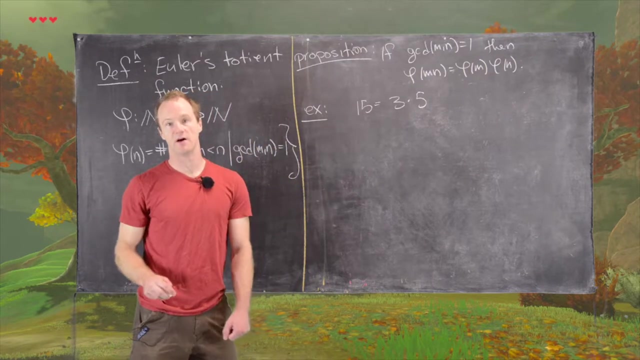 which is 3 times 5.. And again, much like the proof of Euler's phi function evaluated at a power of a prime, we're going to look at an array, So we'll consider the following array of the numbers 1 through 15.. So we'll write it as 1, 2,, 3,, 4,, 5,, 6,, 7,, 8,, 9,, 10,, 11,, 12,, 13,, 14,, 15,, 16,. 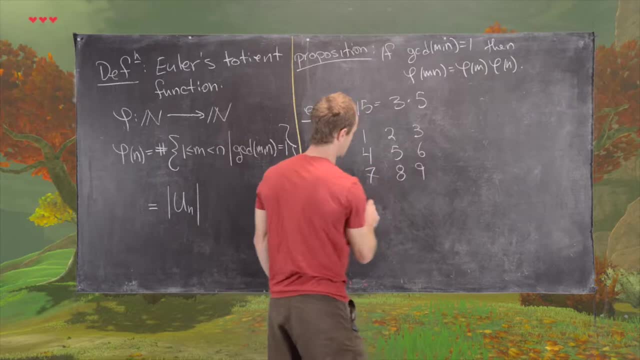 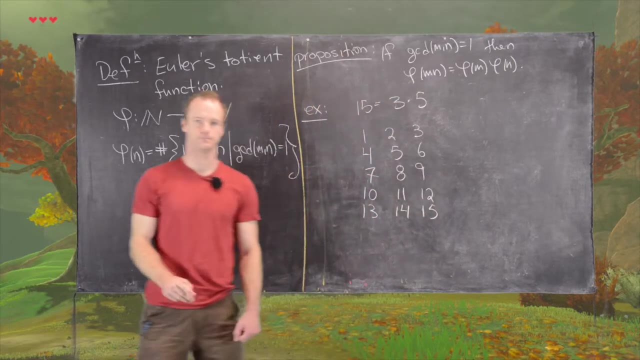 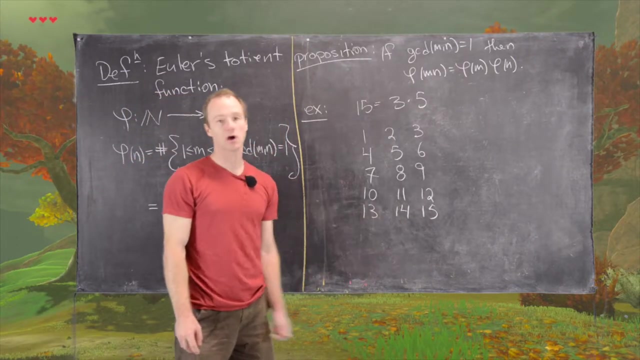 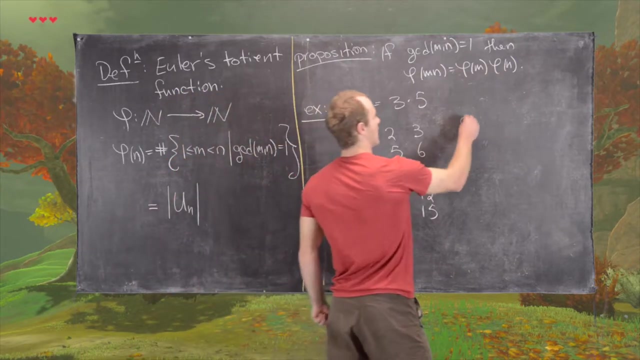 5,, 6,, 7,, 8,, 9,, 10,, 11,, 12,, 13,, 14, 15.. Great, And now what we'll notice is that there are exactly two columns that contain numbers that are relatively prime to 3.. So let's maybe make 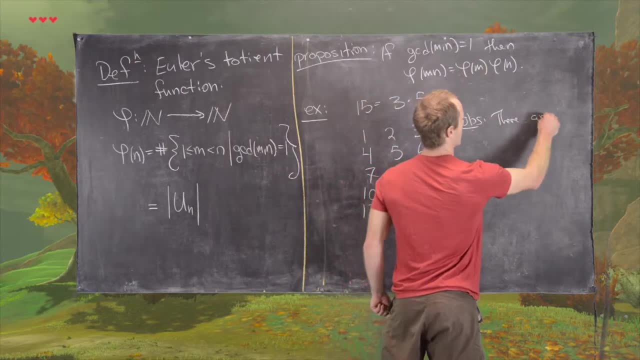 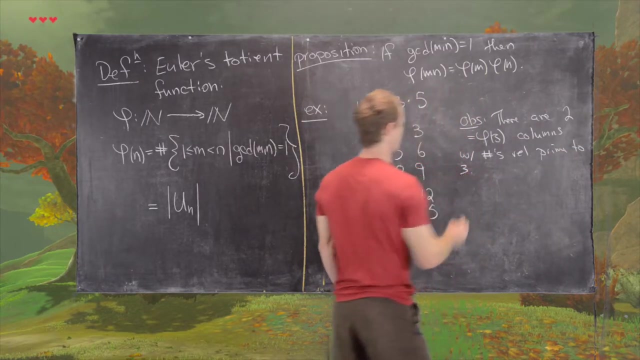 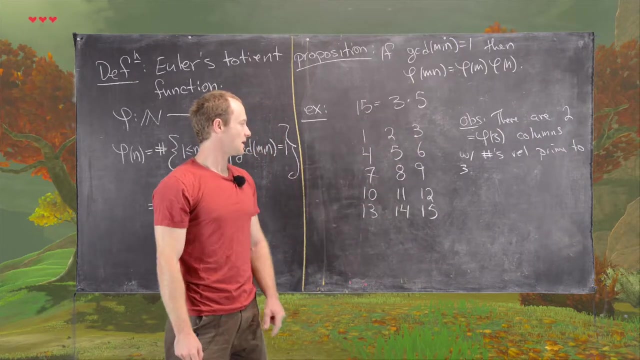 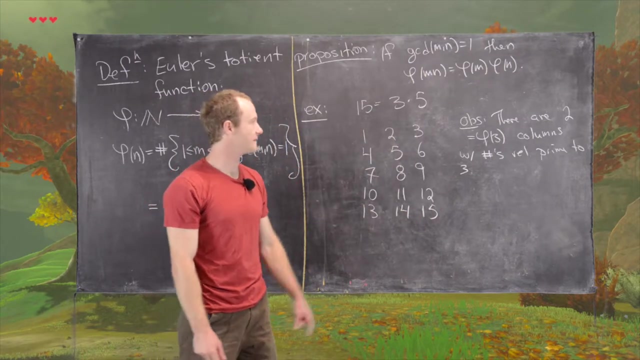 that as an observation. So there are two, Which equals phi of 3 columns with numbers relatively prime to 3.. And that's because each column, each number in the same column has the same residue when you look mod 3.. So everything over here is 0 mod 3.. Everything over here is 2 mod 3.. 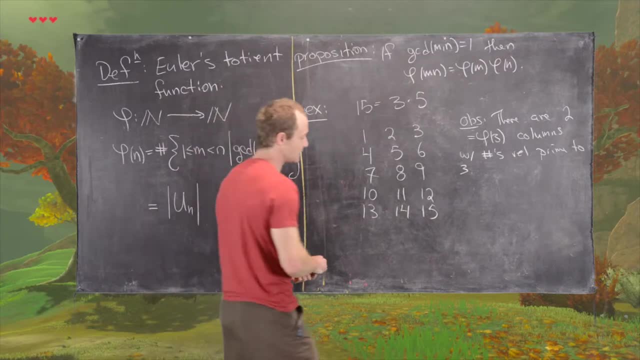 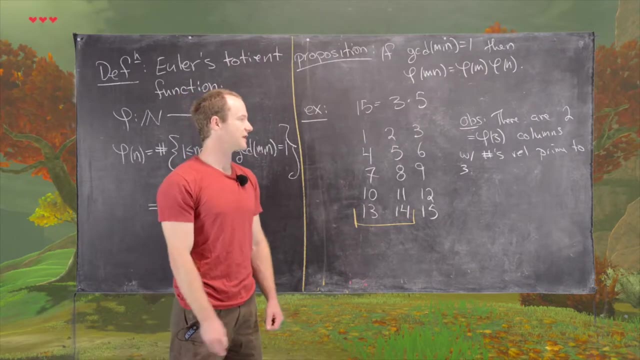 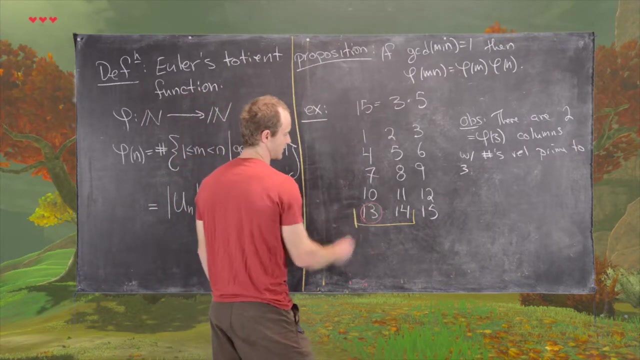 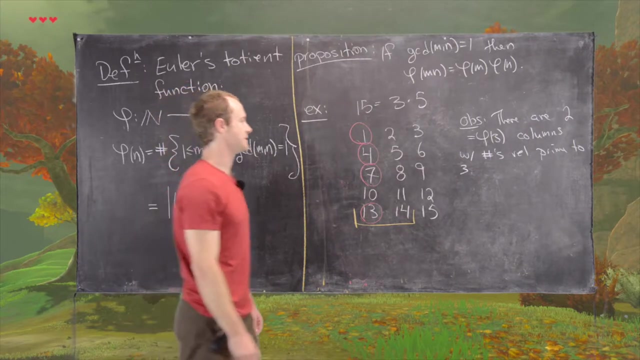 Everything over here is 1 mod 3.. So now, if we restrict ourselves to these two columns and now further look at the numbers in here that are relatively prime to 5, what will we see? So 13 is relatively prime to 5.. 7 is relatively prime to 5.. 4 and 1 are all relatively prime to 5.. And then 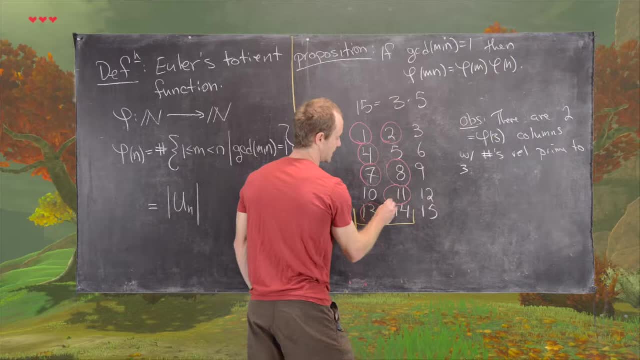 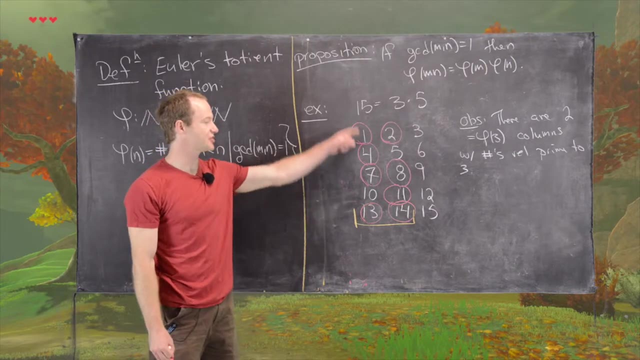 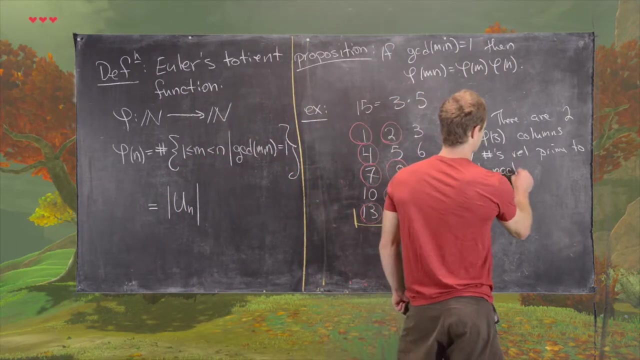 the same thing here: 2,, 8,, 11, and 14.. So let's put that in our observation. So notice that in each of these columns there are 4 numbers that are relatively prime to 5. So in each of these columns there are 4, which equals phi. 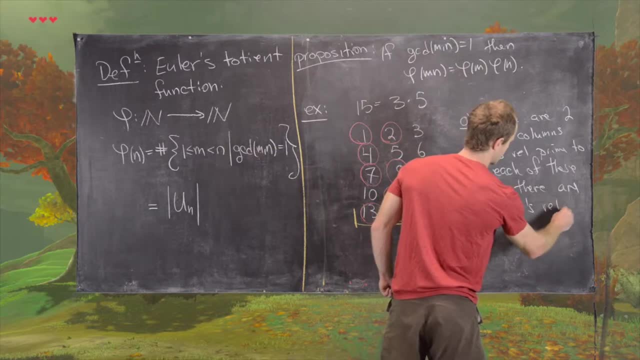 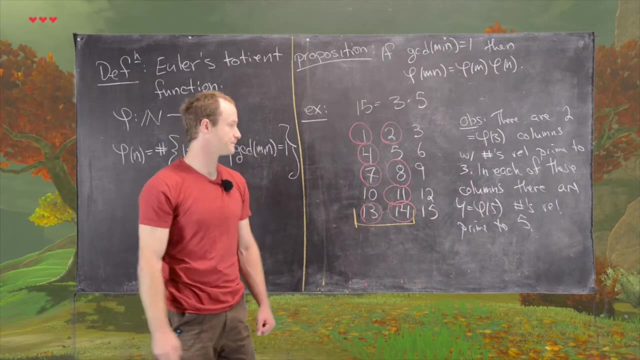 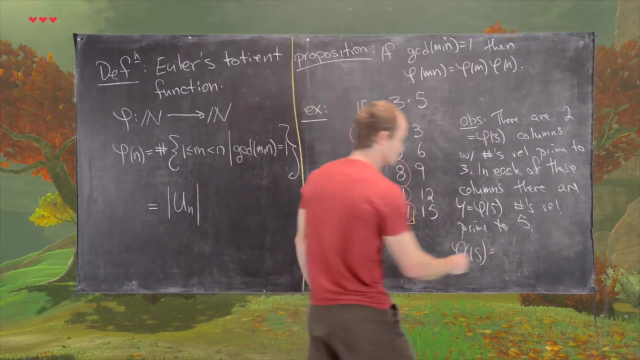 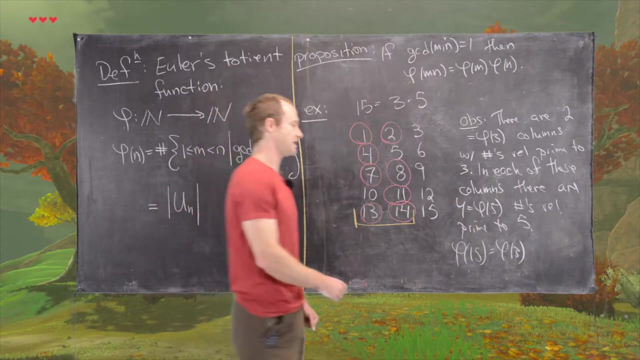 of 5, numbers relatively prime to 5.. Great, And so what that tells us is that phi of 15 you can take by looking at phi of 3, which is each of those columns which are relatively prime to 3, and then multiplying by that. 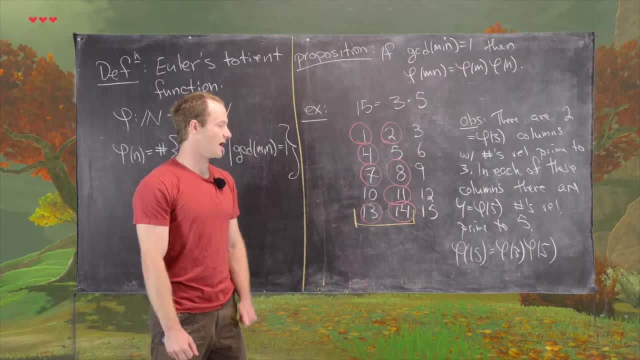 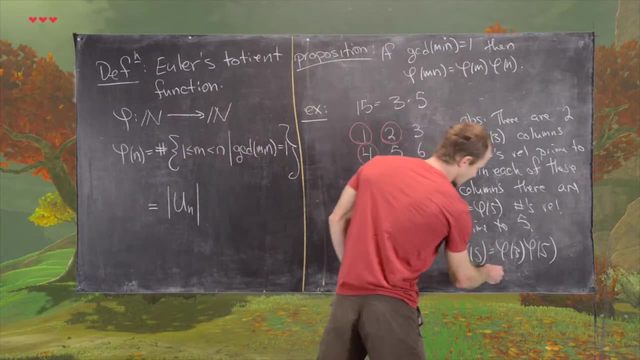 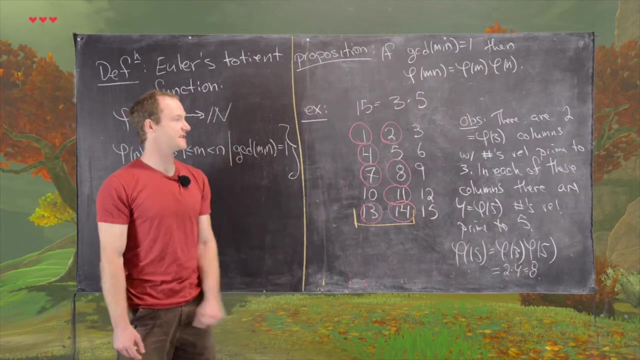 phi of 5, because there are phi of 5 numbers that are relatively prime to 5 in each of these columns. So in other words, we will get 2 times 4, which is 8.. Good, So looking at this example is really informative because it gives us 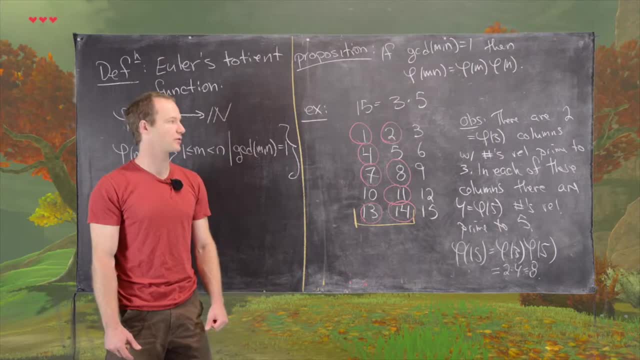 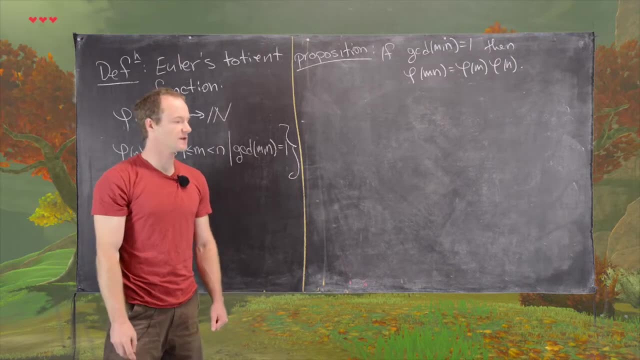 a method for producing a general proof. So let's clean up the board and then we'll look at the proof in general. Okay, now we're ready for the proof in general. So, as was suggested by our example, we'll look at an array of the numbers. 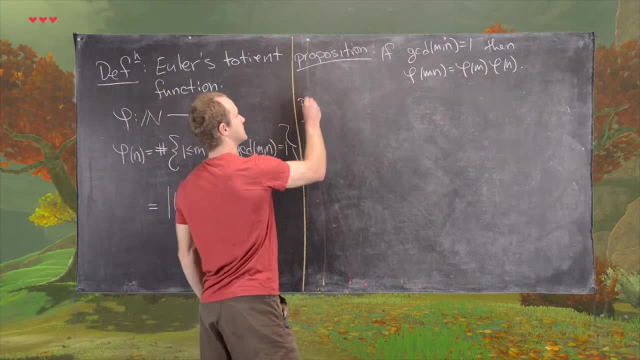 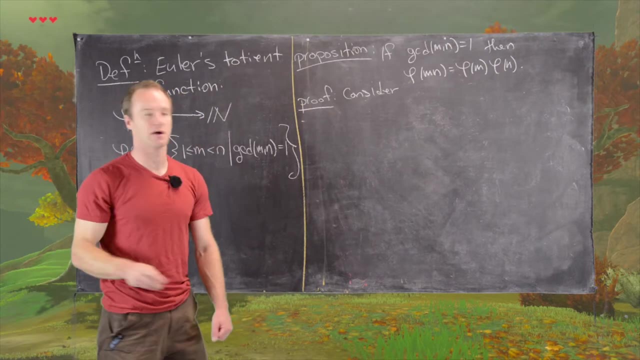 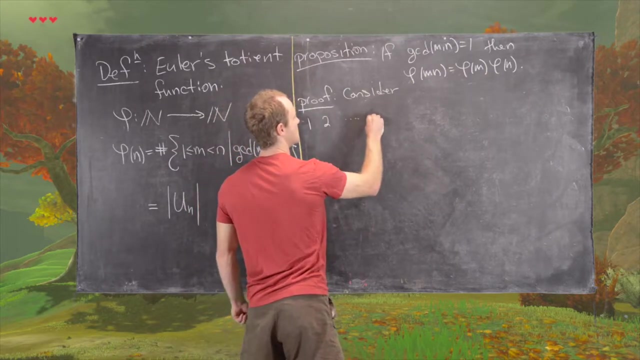 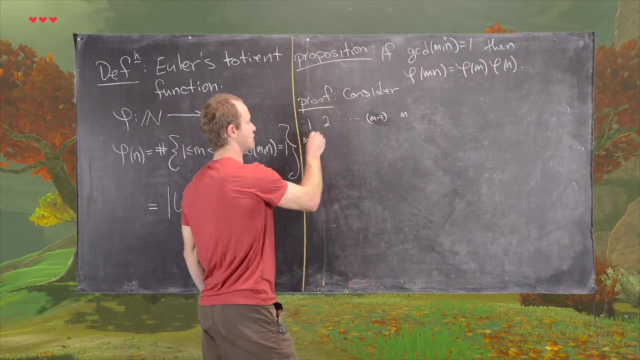 between 1 and mn. So, like I said, let's consider this way of writing the numbers between 1 and mn. So let's do 1, 2, all the way up to mm minus 1 and then m- Good, And then we'll have m plus 1, m. 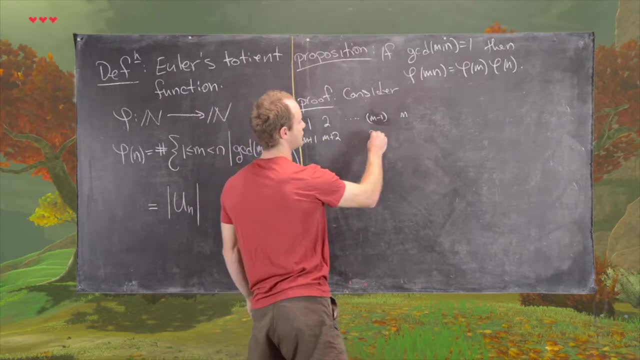 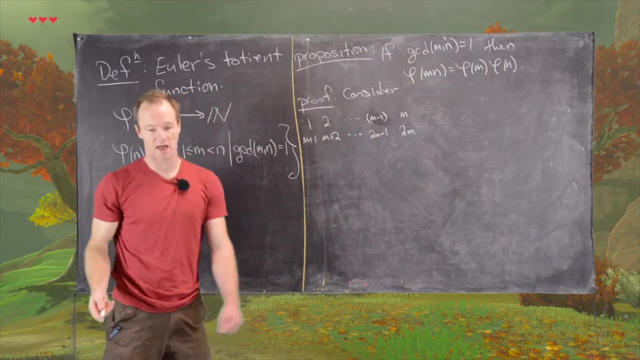 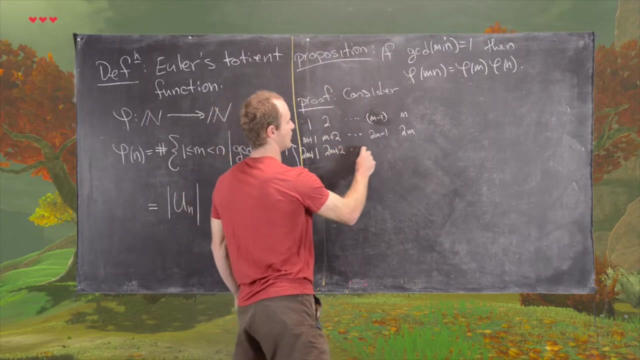 plus 2 all the way up to 2m minus 1.. And then 2m. Good, So, dot, dot dot, And now the next one would be 2m plus 1, 2m plus 2 all the way up to 3m. 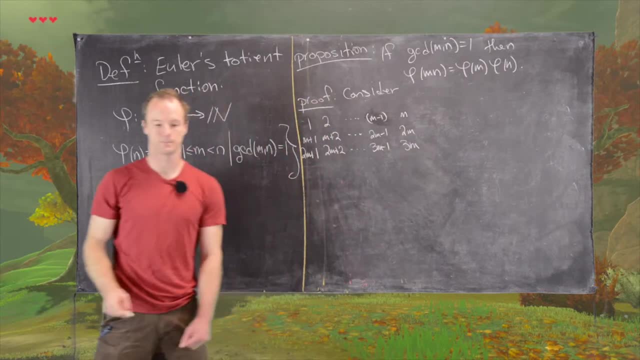 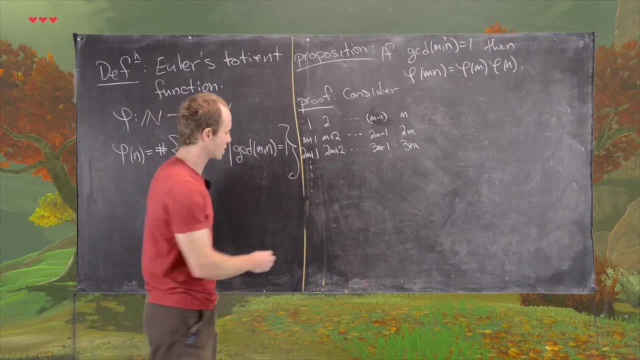 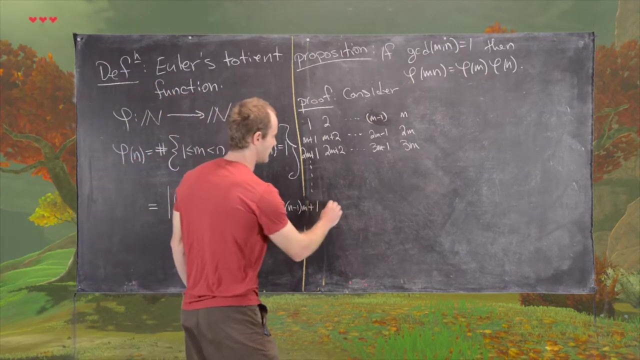 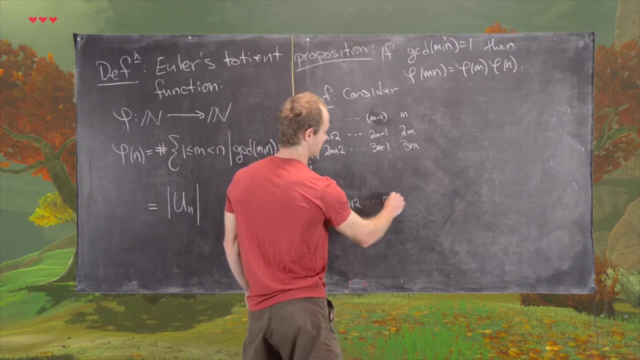 minus 1, and now we have 3m. Okay, now let's go ahead and go down. So down here I'm going to give myself a little bit more room. We have n minus 1 times m plus 1.. Good, And then we have n minus 1 times m plus 2,, all the way up to n times m minus 1, and then n times m. 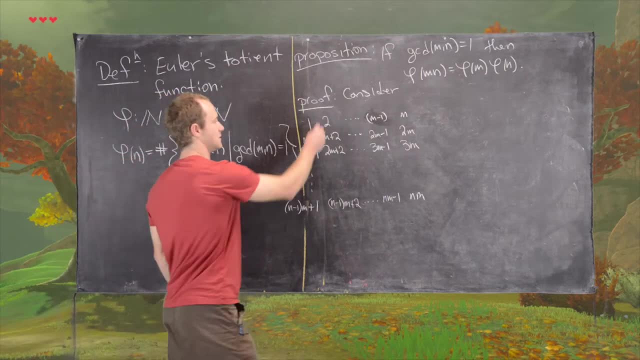 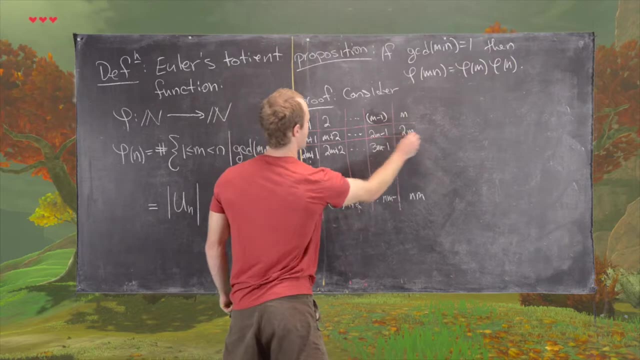 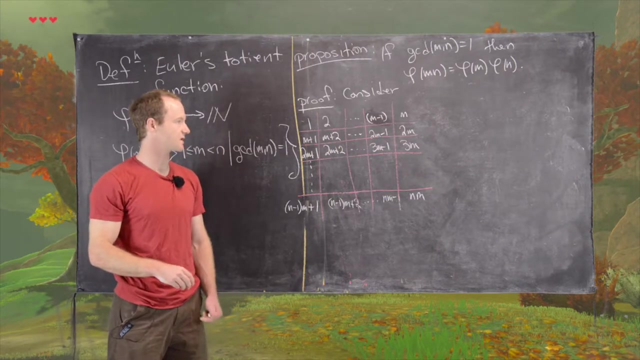 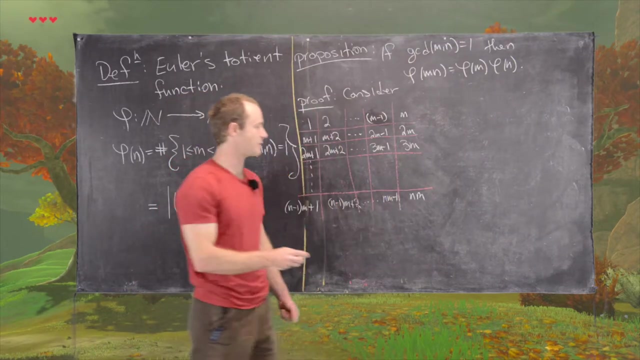 Okay, good. So I'm going to give myself a bit of a grid for this table, so it's easy to see what is where. So now we have a grid for this table, Good. So now what we notice is that in each column, every number has the same remainder when divided by m. 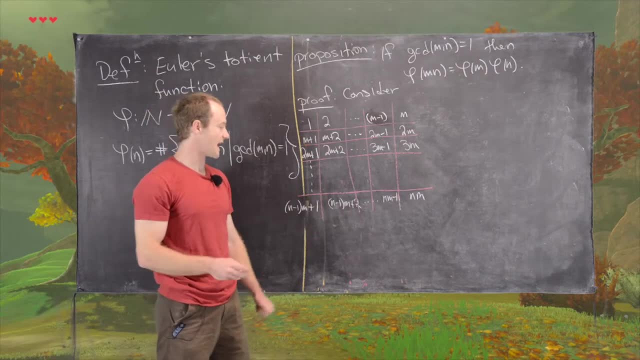 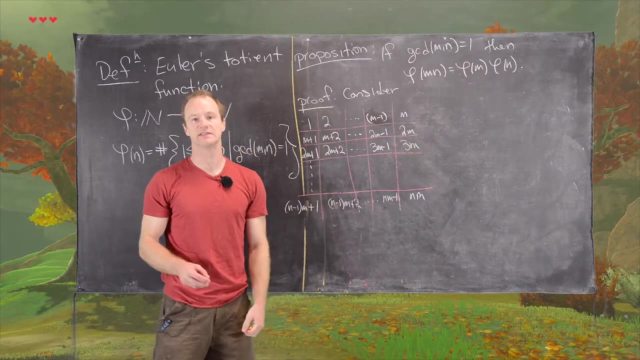 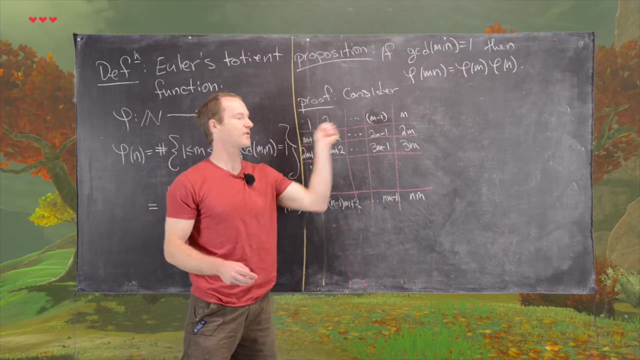 So what that means is that in each column, the GCD of every number in the column with m is the same, And so that means all we need to look for is the GCD of the number. So we're going to look for the numbers in the first row in order to find the GCD of the numbers all the way down. 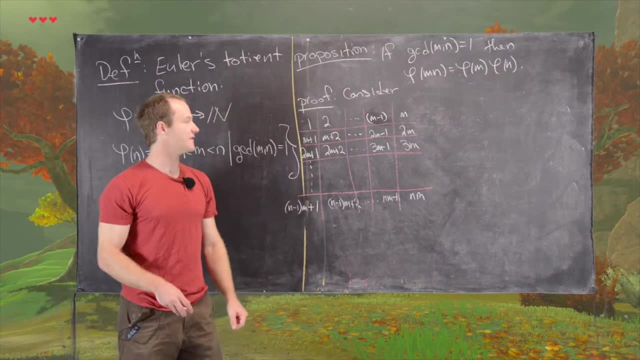 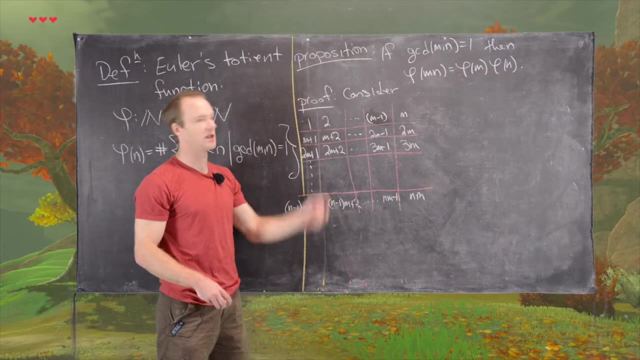 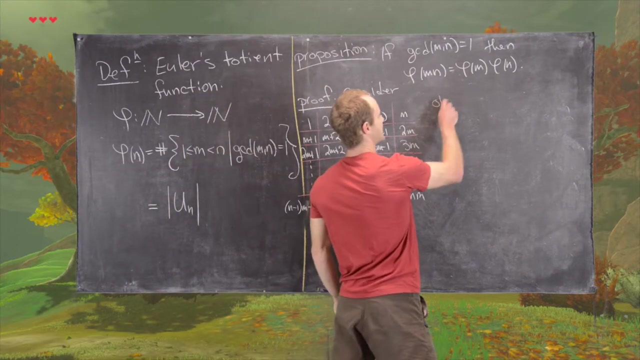 And we know that among the first row, phi of m of them are relatively prime to m, and so that we have phi m columns that are made completely of numbers relatively prime to m. So let's maybe make that an observation. So there are 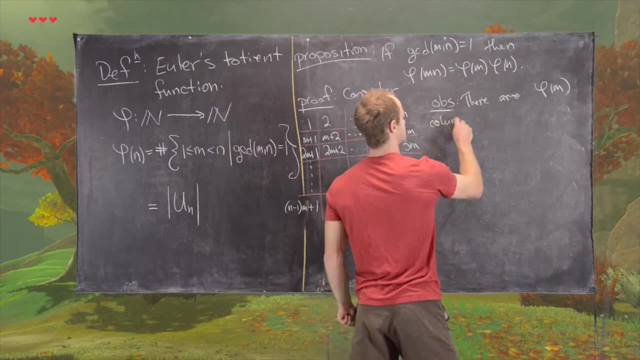 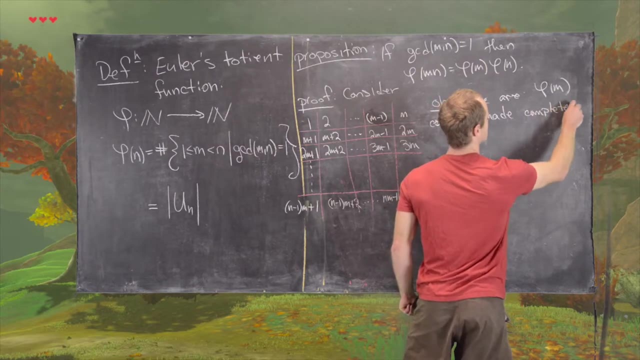 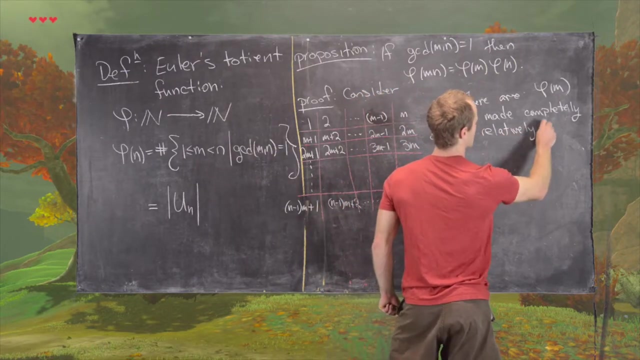 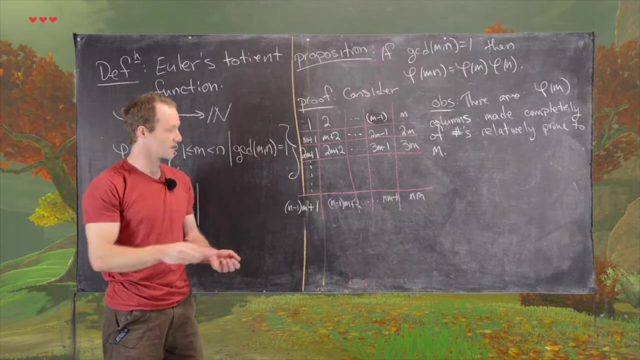 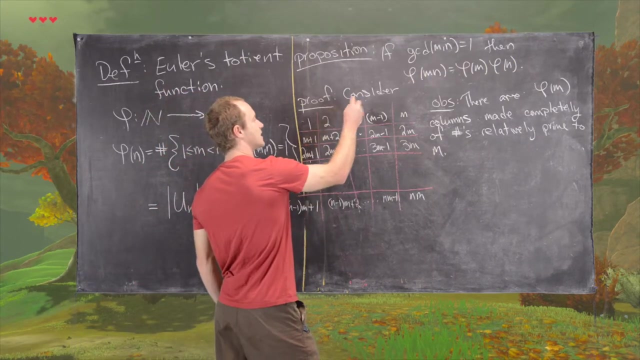 m columns made completely of numbers, relatively prime to m. Good. So let's say we have one of those columns and let's like sneak it in right here so we could have m plus k would be the column right there. Well, actually, maybe we would say this was k right here, then it would be m plus k right here. 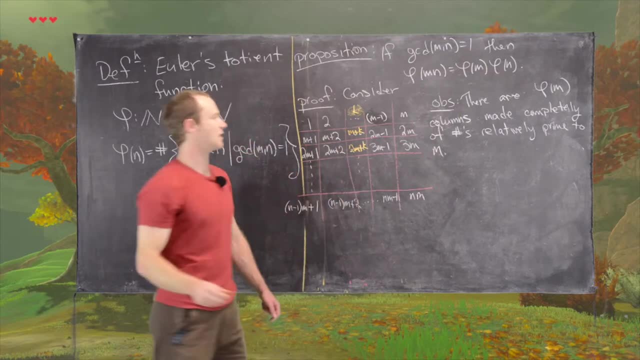 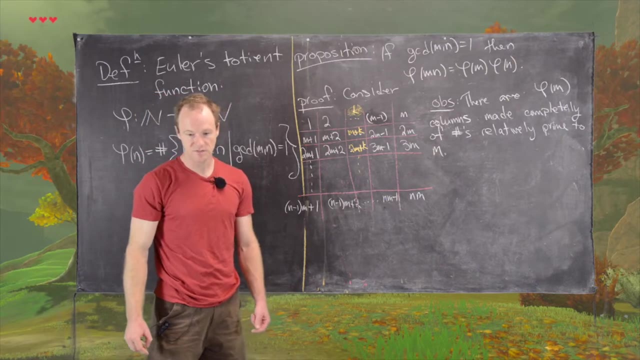 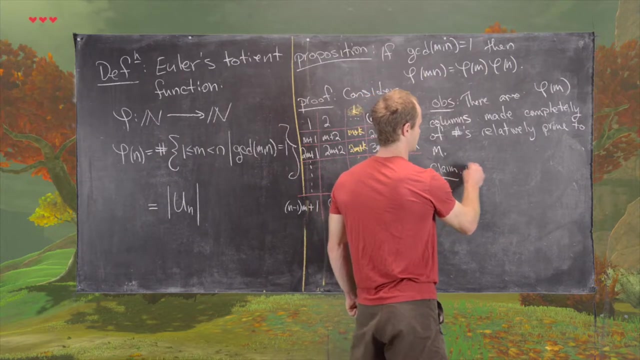 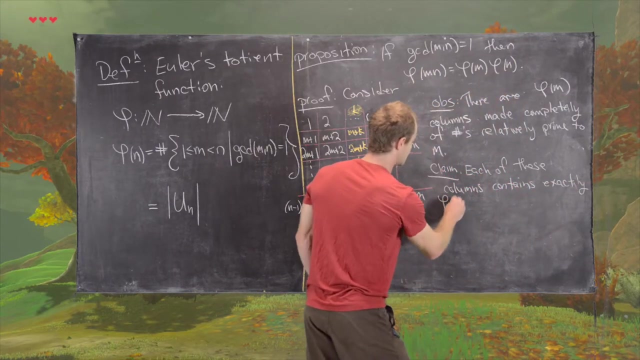 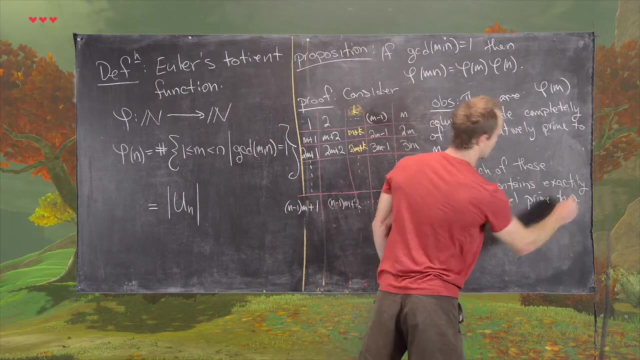 2m plus k right here and so on. So that would be one of the columns that's relatively prime to m Great. So now here's our next claim. Each of these columns contains exactly phi to the n numbers relatively prime to n. 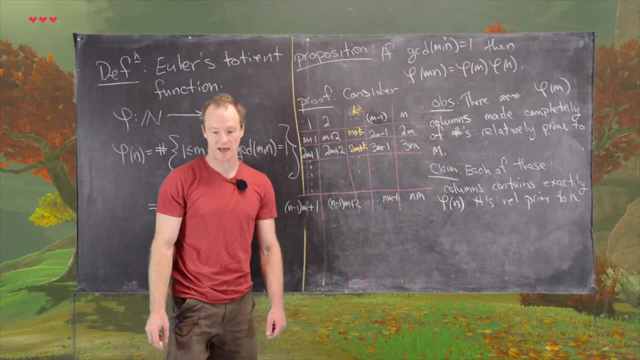 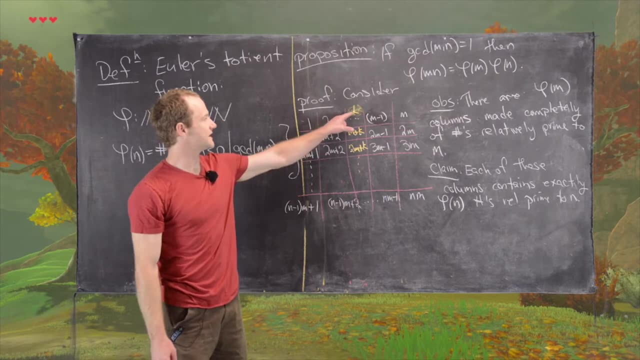 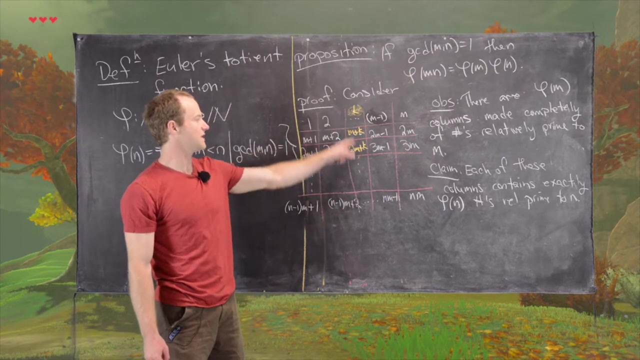 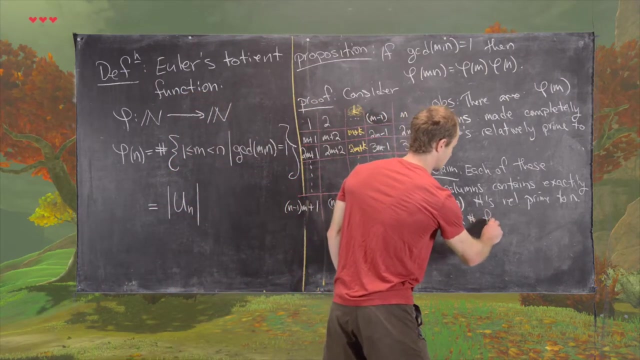 Good. So let's see how we could do that. So we could do that by the following: So we'll look at this column k and now notice, let's take two entries from column k, So take two numbers from column k. 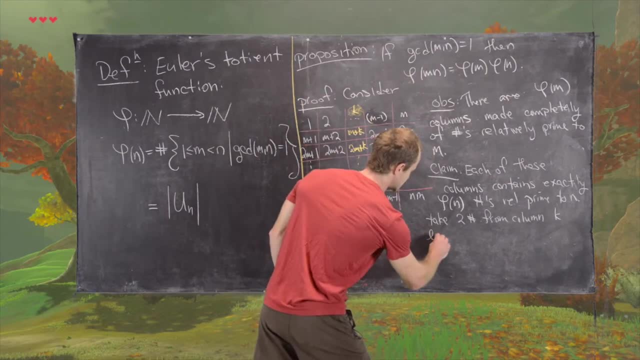 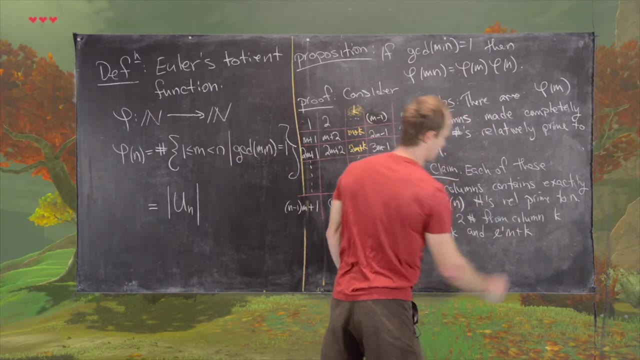 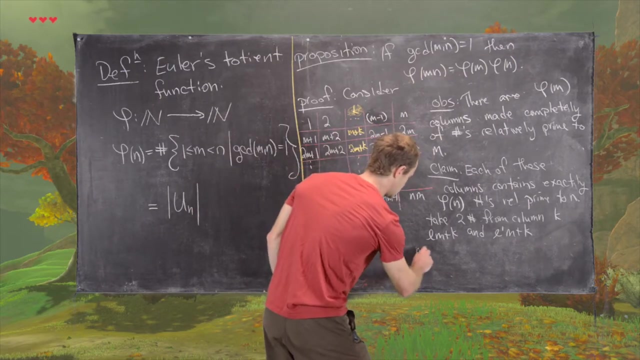 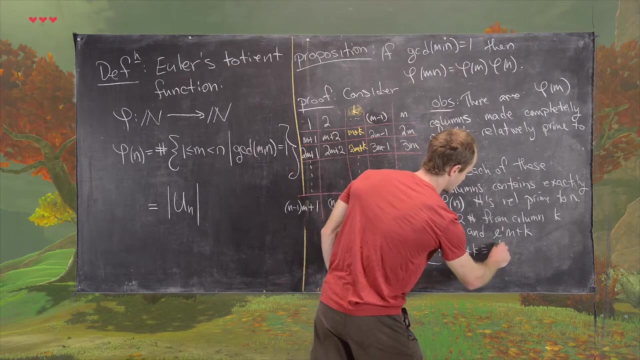 Okay, So let's say we have l times m plus k and l prime times m plus k. Good, And let's notice, Notice the following- that l times m plus k is congruent to l prime times m plus k, mod n. 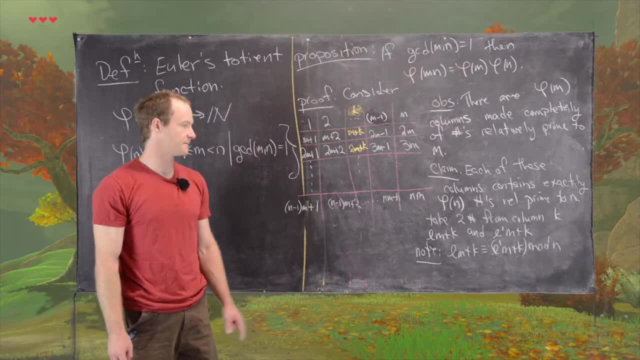 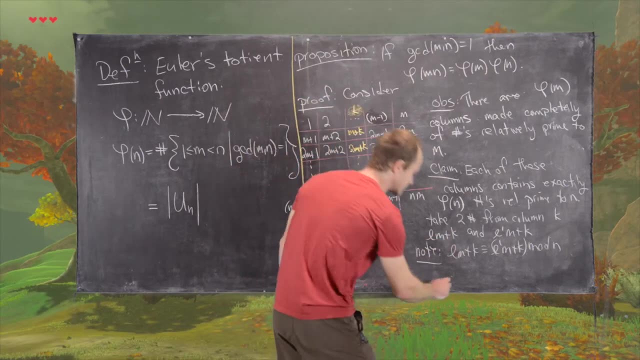 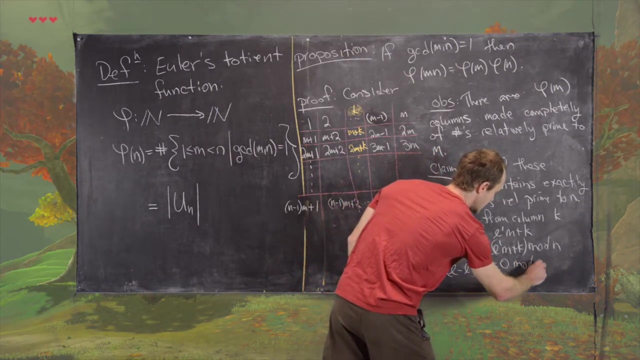 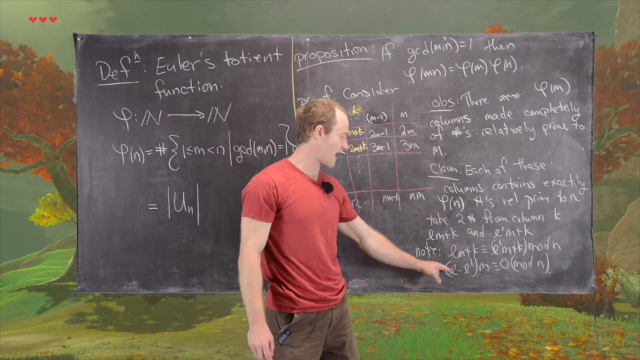 Okay, So let's see why that's the case. And so that's true, because if we were to subtract this, this statement is equivalent to l minus l. prime times. m is congruent to 0 mod n. Good, But that tells us that n either divides m, which we know, that n does not divide m. 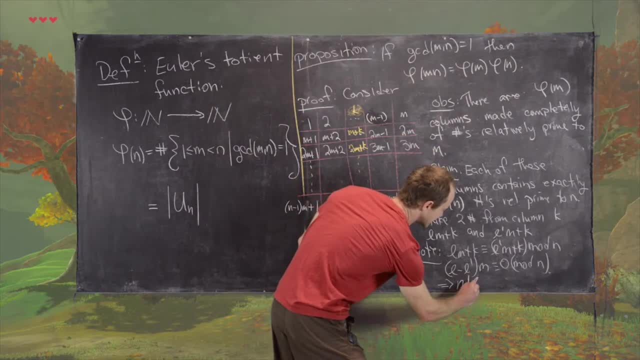 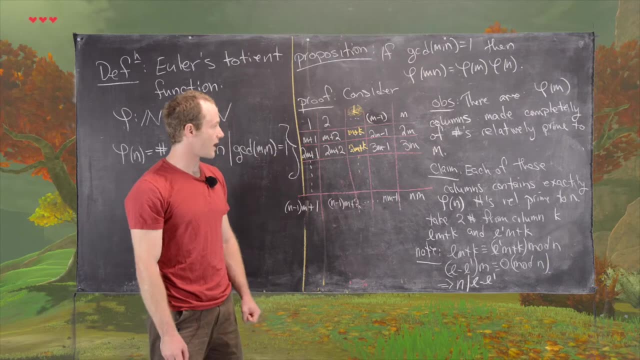 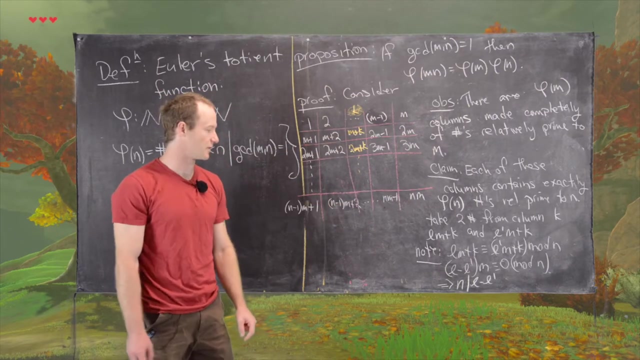 but that tells. So that tells us that n must divide l minus l prime. Good, But now, since l and l prime are only between 0 and n minus 1, so notice, this is the n minus 1 row, so 0 and n minus 1, that means l has to be l prime. 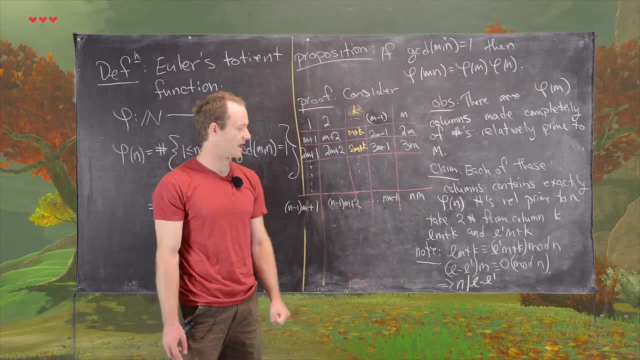 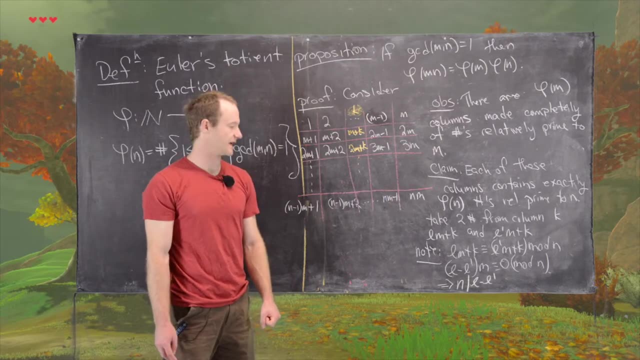 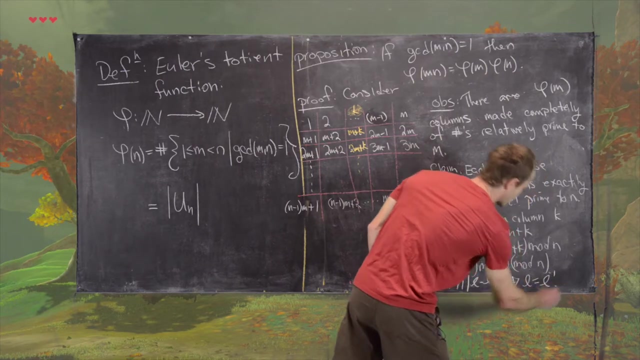 Because what we're getting here is l minus l prime is a multiple of n, but l and l prime are not, are not allowed to be big enough to produce a multiple of n, except for the zeroth multiple of n. So what that tells us is that l is equal to l prime. 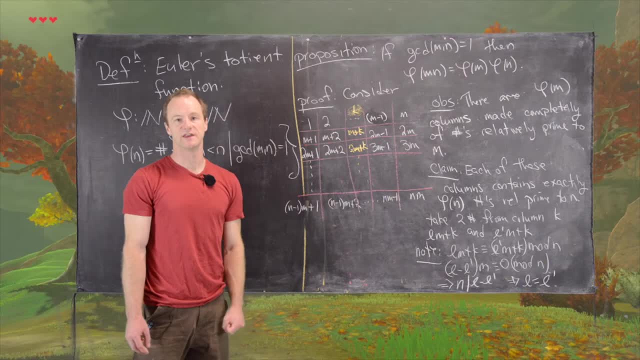 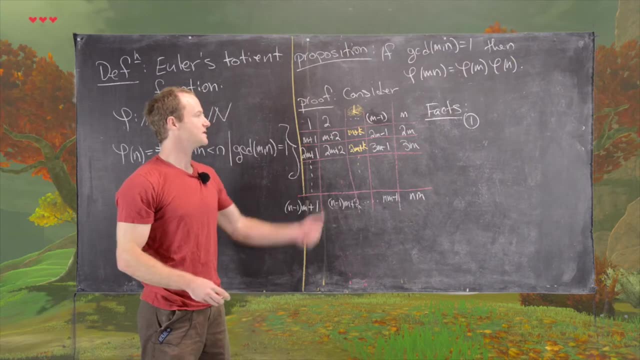 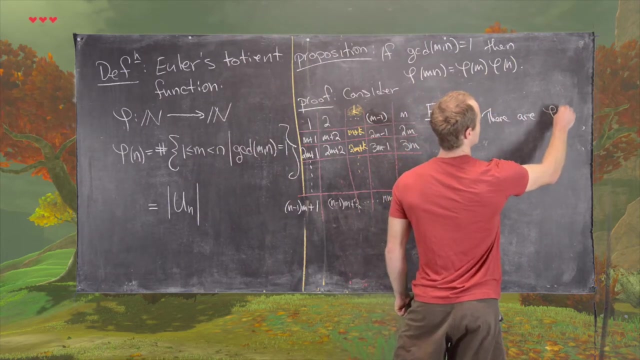 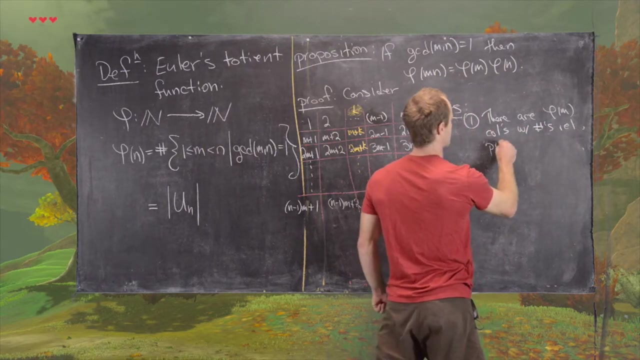 Okay, Good, So I'll clean up this a bit and then we'll finish it all off. Okay, So let's just summarize the facts that we have so far. So fact number one is: There are phi m columns with numbers relatively prime to m.